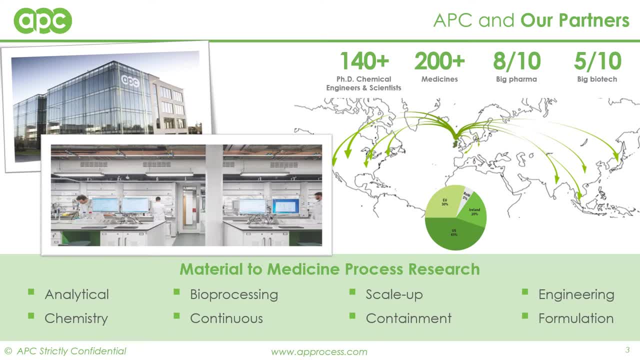 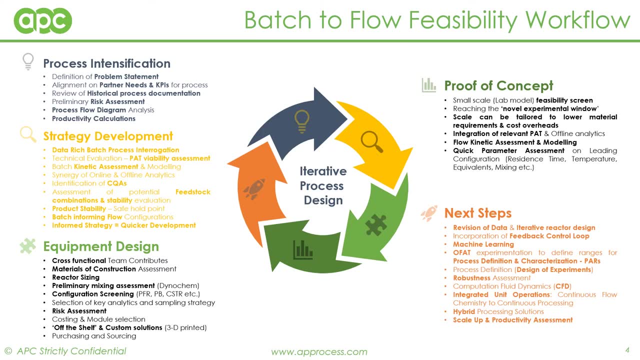 can be developed by developing the data and then, as a result, provide the opportunity for and characterization so our partners can accelerate the development process. the advantages to implementing flow chemistry and continuous processing configurations are well documented. these advantages include increased safety, increased quality, such as yield impurity. these increased qualities are often 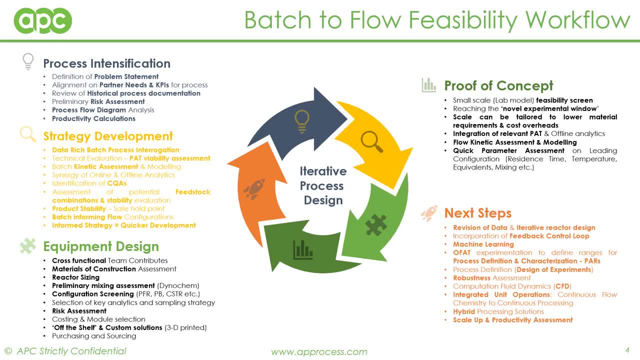 achieved by reaching the novel experimental window enabled by flow chemistry, the integration of unit operations, increased productivity, and all while reducing that all-important footprint. APC employs an iterative process design strategy to enable process intensification by the conversion of batch processes to flow. our teams of scientists and engineers 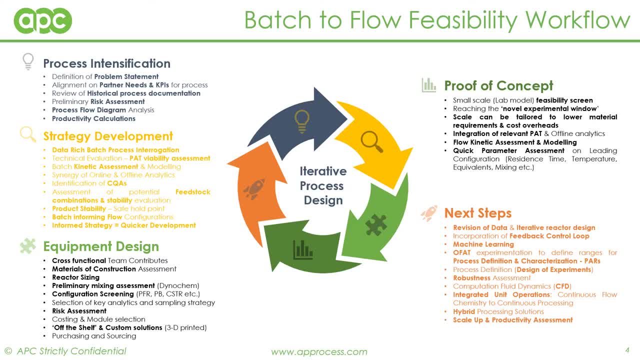 utilize this framework to move from concept onwards towards strategic planning and design, to proof of concept and eventually onwards to the next generation: an informed conversion strategy and design. elaspen to move swiftly to proof of concept. work with integrated Pieten offline analytics on a range of in-house 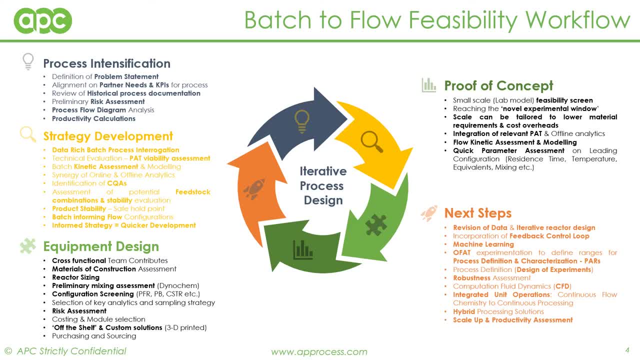 screening platforms, with both custom and off-the-shelf solutions. of course, depending on the face of the molecule in development phase, appropriate work packages can be added or subtractive. following are successful proof of concept. the next steps would include the integration of unit ops feedback control. 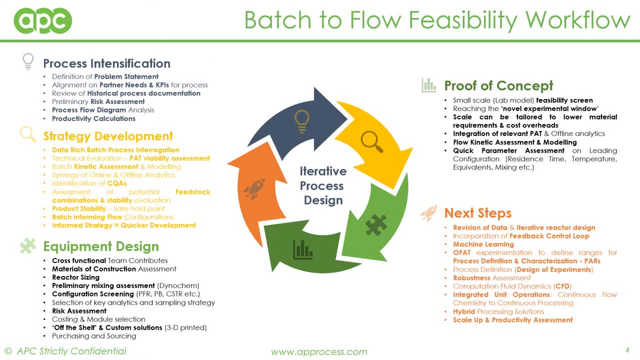 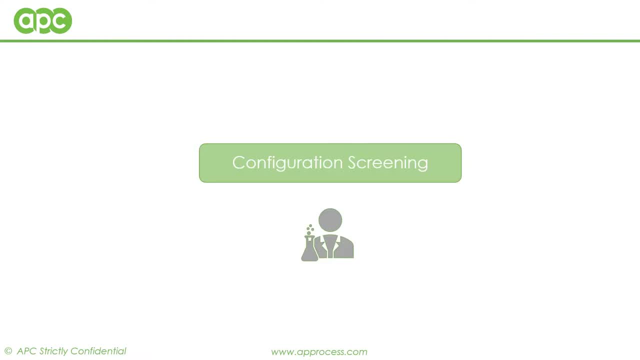 machine learning, design of experiments or the development of hybrid solutions, depending on the needs of our partner. Over the next section- configuration screening- I am going to take you through some of the aforementioned steps we typically employ while taking that leap from batch processing to continuous processing. 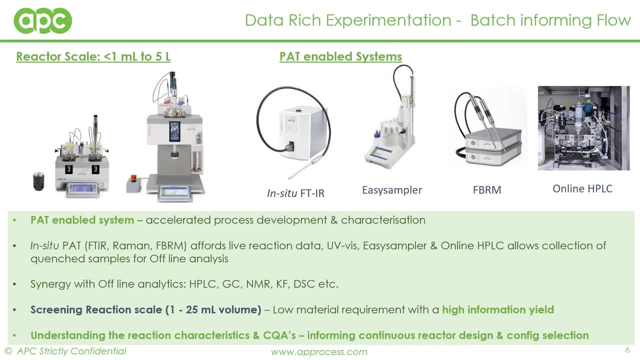 Data rich experimentation is key to our approach here at APC, in batch and in flow. but more importantly in our case, for batch informing flow, We must understand the reaction characteristics, the critical quality attributes, and this will help us inform the continuous reactor design and configuration selection. I suppose APC chemists are a little bit different. we are 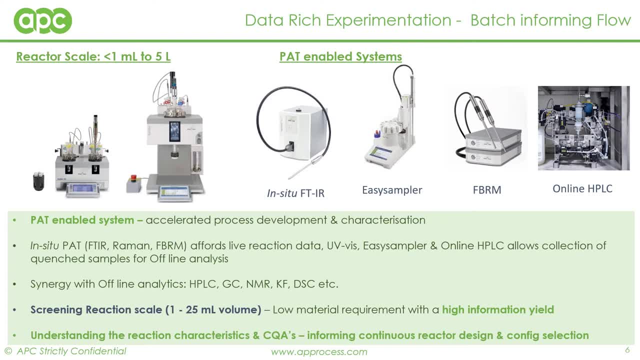 trained in the use of PAT enabled systems, which allows us to accelerate that data mining process and characterisation of reactions. The targeted use of PAT, combined with our in-house expertise of chemistry engineering, affords data rich experimentation, which really means you get a higher yield of information. 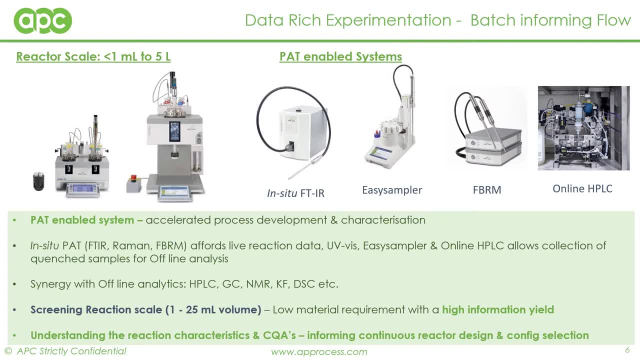 per experiment. The application of FTIR, RAM and FPRM affords live reaction data allowing us to track catalytic reactions, heterogeneous or homogenous reactions, and easily characterise these. We can screen from 1mm to 25mm scale, and this 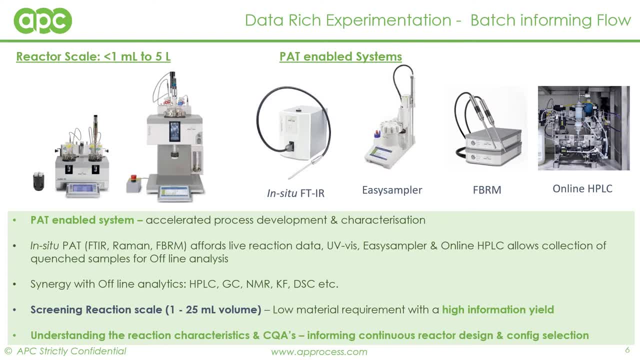 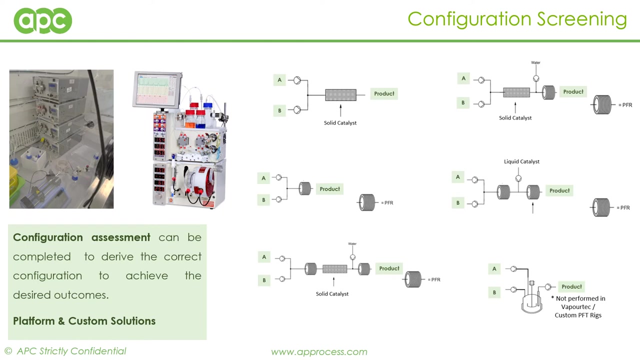 is really attractive. It is this information that we then feed into the next stage, which is configuration screening, Following our batch process, technical assessment. we now know how our chemistry performs. Is it homogenous or heterogeneous? Does it use a catalyst? Is it mixing limited? How quickly does it reach completion? 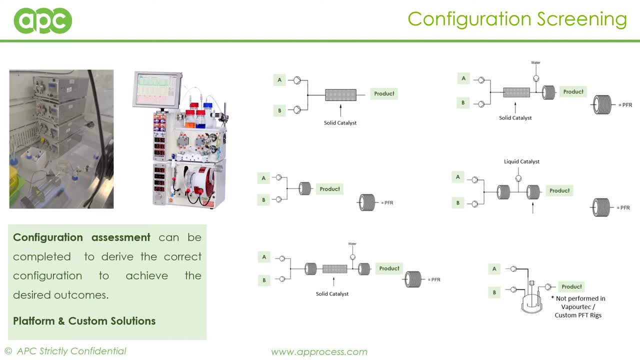 We have most likely trialled FTIR, RAM and UV or LC as online methods of characterising and following this reaction. All these factors and the data collected influence reactor design and selection, whether that be PFR, packed bed, CSTR or a combination Configuration. 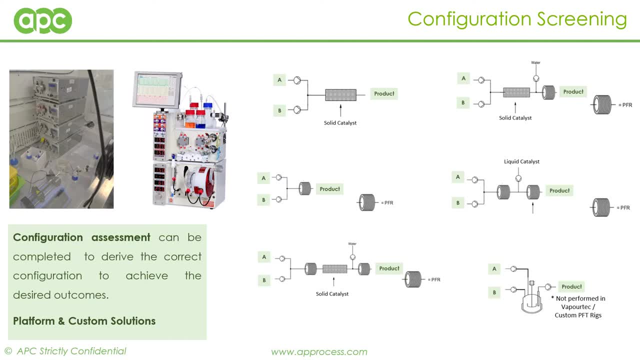